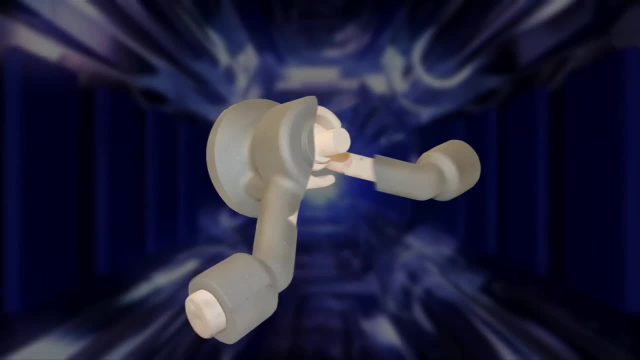 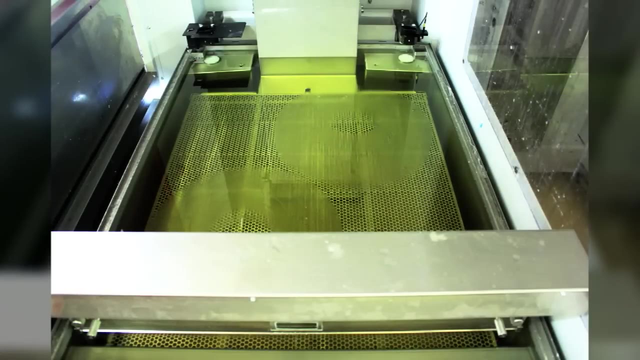 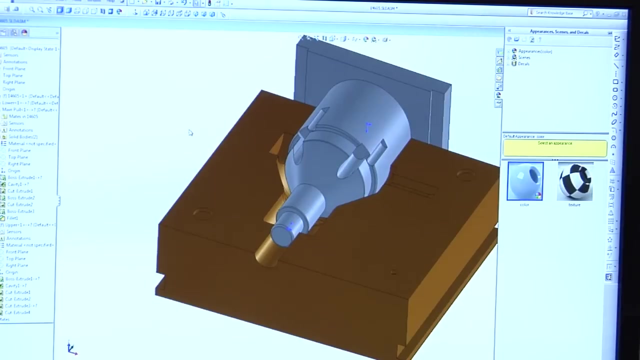 wax or ceramic coring techniques for more complex internal detail, For prototyping or very short runs. purchasing of production-oriented tooling is not always economical, so we offer the option of special printed patterns produced using stereolithography from 3D CAD data. 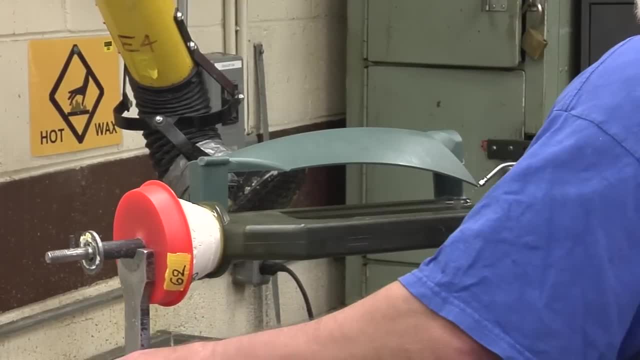 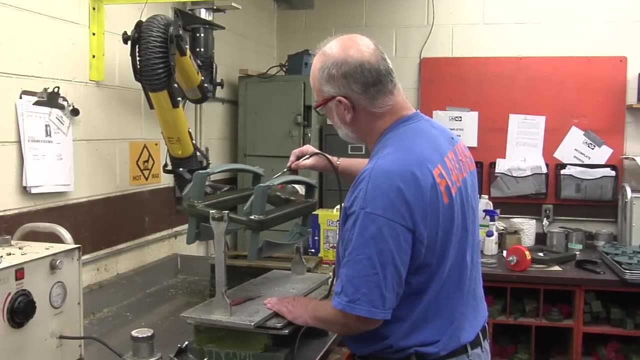 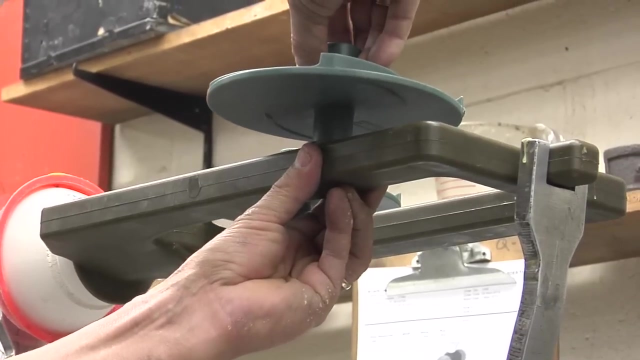 Once the wax patterns are produced, they must be assembled to a feed system called a sprue. The sprue is made from reclaimed wax and designed to not only hold the wax patterns but also engineered to form a sufficient pathway. Metal flows through the mold during casting to produce a sound and defect-free component during solidification. 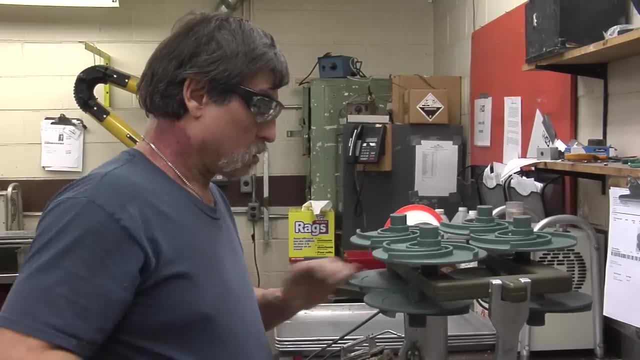 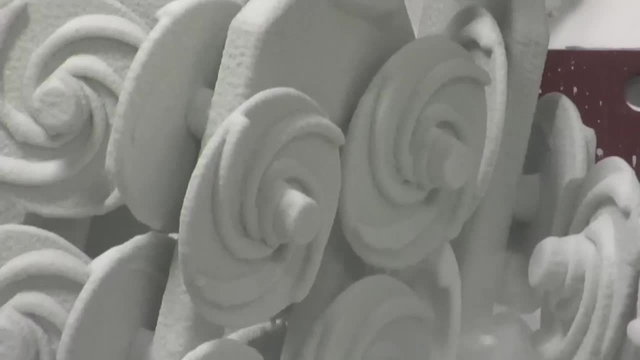 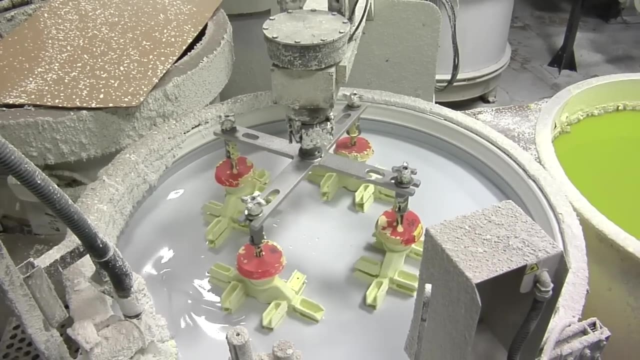 With the waxes now assembled to the sprue, we have completed what is called a tree. To transfer the exact detail of the wax pattern to the casting, the trees are encased in a seamless ceramic shell mold. It is formed by robots dipping or investing the wax into a slurry, drying the tree and repeating. 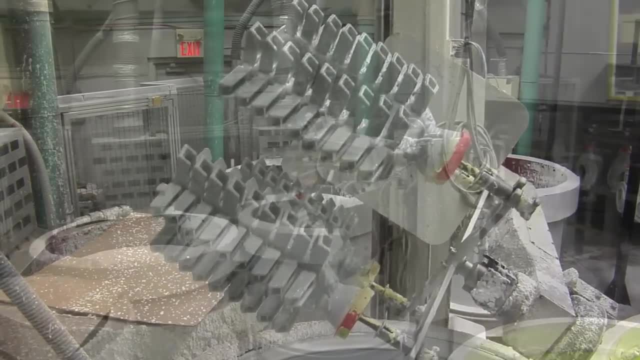 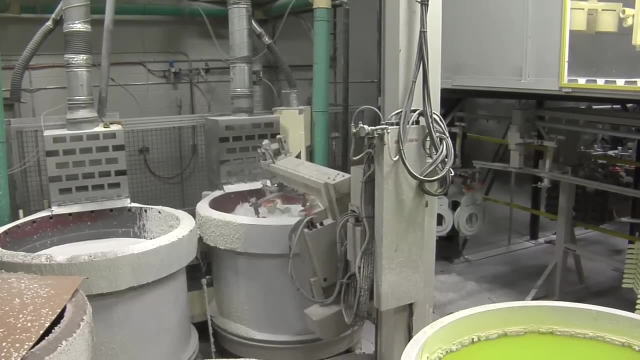 This builds up three-eighths to one-half inch of ceramic around the tree. It is this ceramic shell or mold which will receive the molten metal during casting. The first coat is called the primary. It forms the innermost surface of the mold. 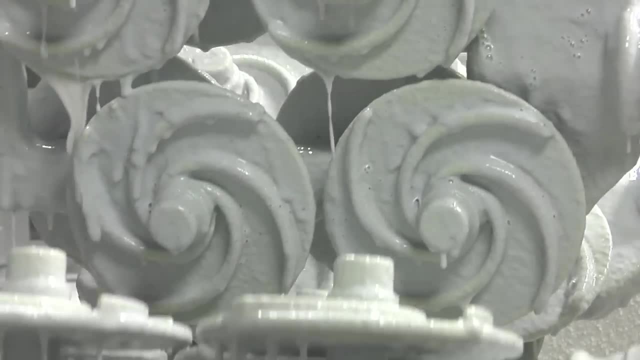 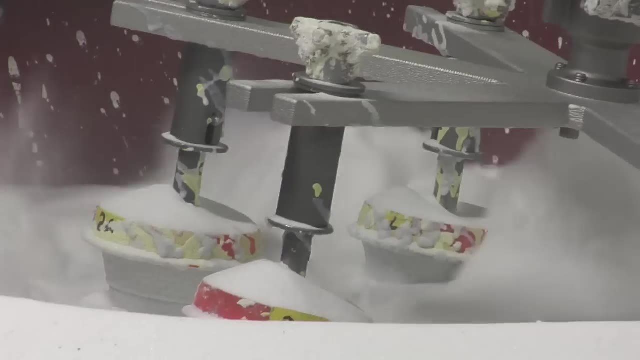 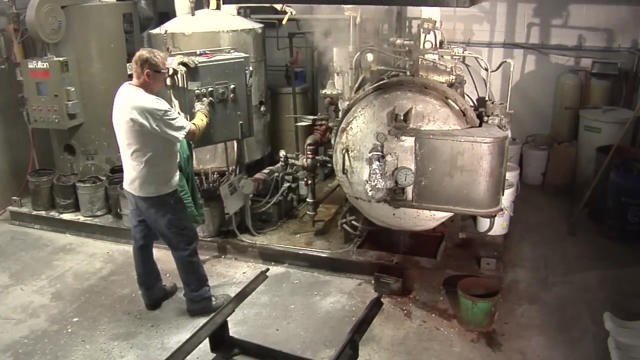 For that reason it must be carefully applied in very controlled conditions to ensure the quality. Gradually, additional layers of increasingly coarser secondary ceramic layers are added and the completed shell takes form. The next step is to remove the wax patterns and sprue. 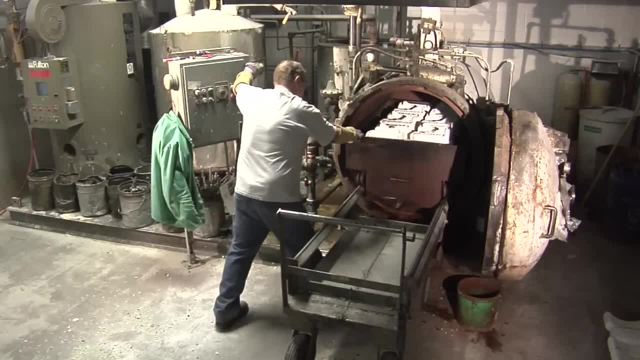 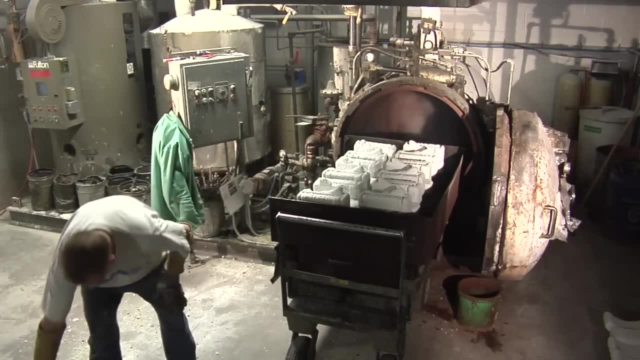 We do this by inverting the shell into either a steam autoclave or flash-fire de-waxing furnace. The wax melts and runs out, and the shell is now complete and fully self-supporting. When the shells are scheduled to be poured, 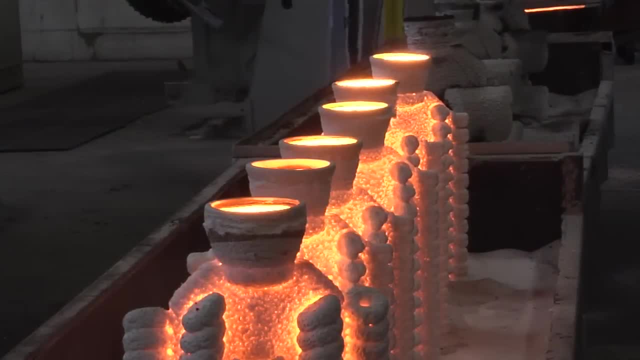 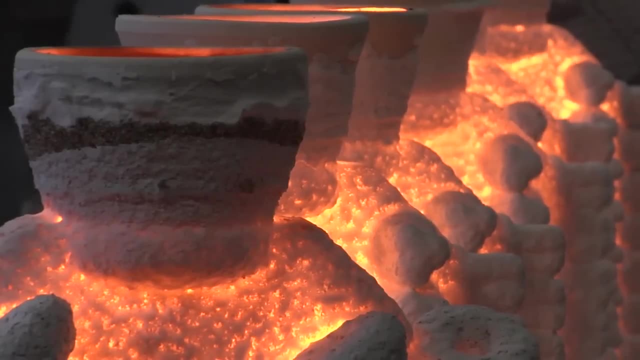 they are reheated to approximately 1700 degrees to further condition and strengthen the ceramic shell. They are now able to withstand the thermal stress they must endure. during the next stage, While the shells preheat, we prepare and melt the metal to be cast.